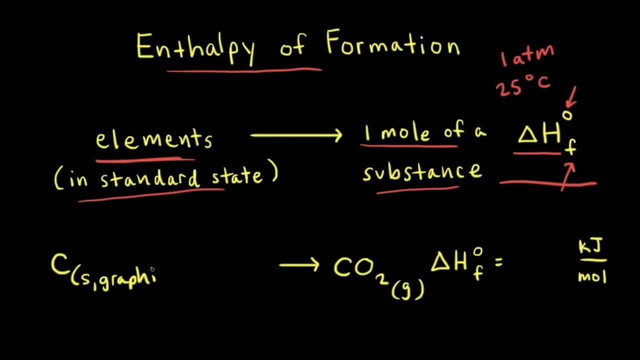 and we're gonna write graphite over here And next. when you think about the most stable form of oxygen under standard conditions, And so at one atmosphere, so atmospheric pressure and room temperature of 25 degrees Celsius, the most stable form of oxygen is oxygen gas. 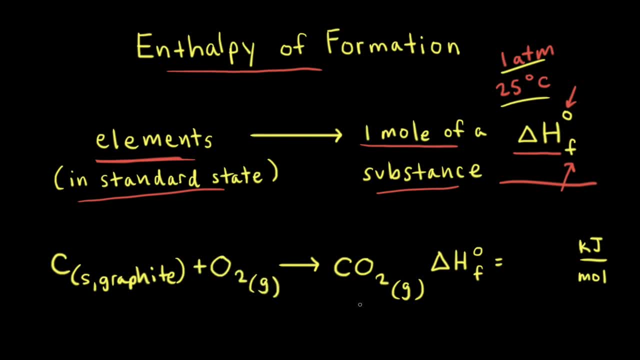 So we can go ahead and write in here O2.. And since we're forming one mole of carbon dioxide from the elements that make up carbon dioxide in their most stable form under standard conditions, the change in enthalpy for this would be the standard enthalpy of formation. 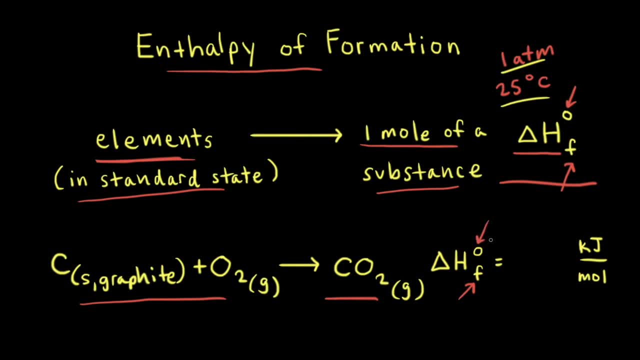 So we have our subscript F and our superscript not to indicate standard conditions. The change in enthalpy for the formation of one mole of CO2 is equal to negative 393.5 kilojoules per one mole of carbon dioxide. Let's look at some more equations showing the formation. 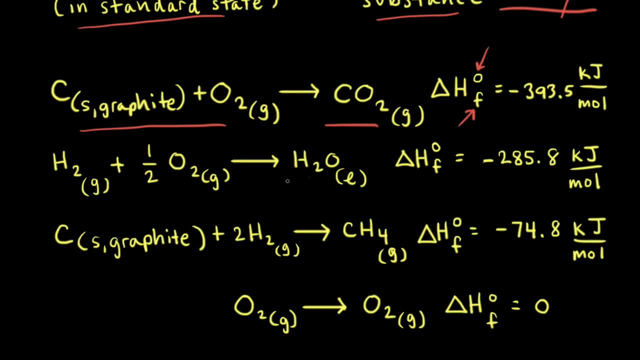 of one mole of a substance. For example, let's look at the equation showing the formation of one mole of water. So water is composed of hydrogen and oxygen, and the most stable forms of those two elements under standard conditions are hydrogen gas and oxygen gas. 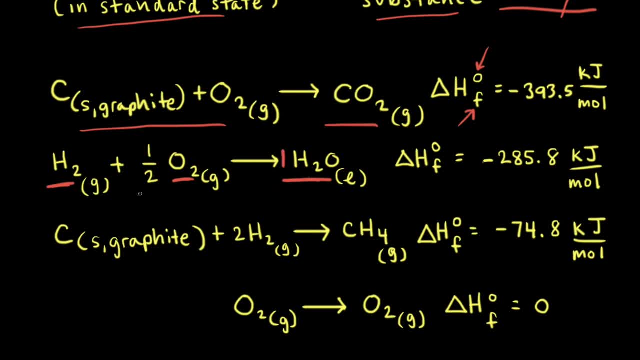 And for the coefficients: to make one mole of water we need a one half as our coefficient in front of O2.. The standard change in enthalpy of formation for the formation of one mole of water is negative 2.5.. So we're gonna write that down. 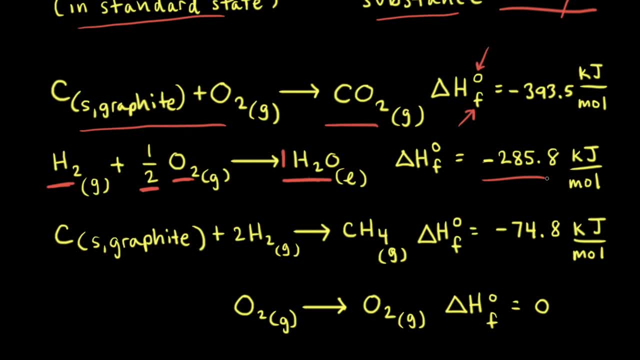 So we have 285.8 kilojoules per mole. We can do the same thing for the formation of one mole of methane, CH4.. We already know that the most stable form of carbon is graphite and the most stable form of hydrogen. 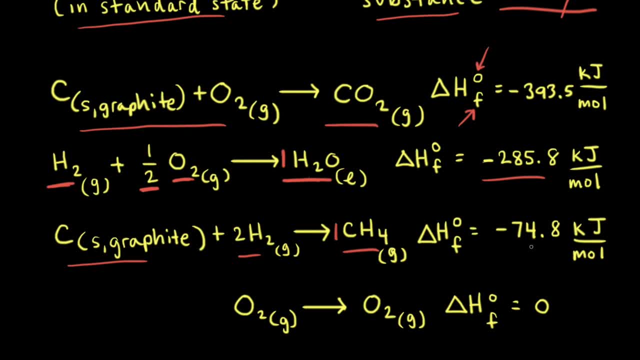 is hydrogen gas, And the standard change in enthalpy of formation for the formation of one mole of methane is equal to negative 74.8 kilojoules per mole. Next, let's think about forming one mole of oxygen gas. Well, we're forming the oxygen gas, right? 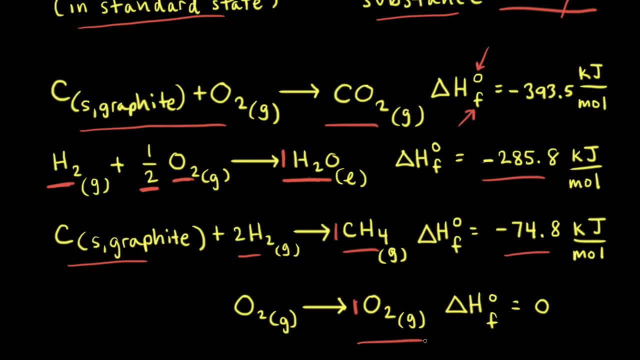 We're forming the oxygen gas from the most stable form of oxygen under standard conditions, which is also diatomic oxygen gas: O2.. So we're not changing anything. We're going from O2 to O2.. And since there's no change, there's no change in enthalpy. 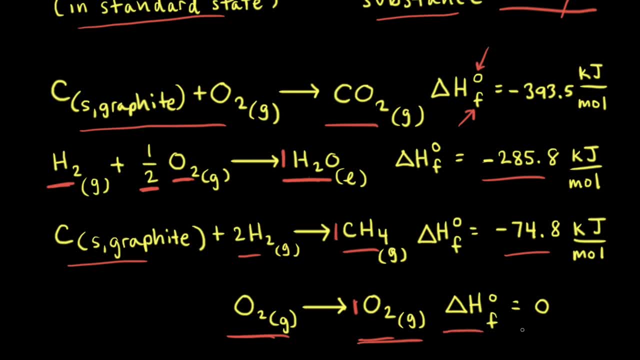 Therefore, the standard enthalpy of formation is equal to zero, And this is true for the most stable form of any element. The standard enthalpy of formation of the most stable form of any element is zero, since you'd be making it from itself. 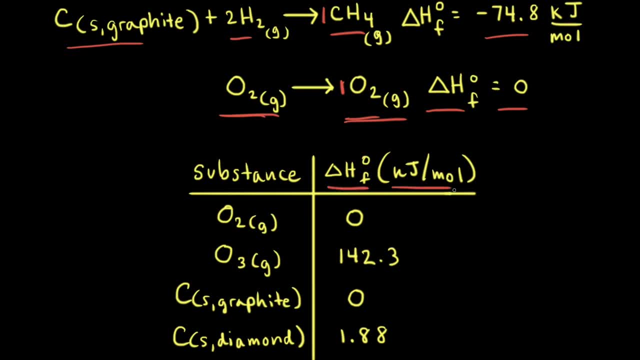 Standard enthalpies of formation of one kilojoules per mole are often found in the appendices of many textbooks And if you look in the appendix of a textbook you'll see. the standard enthalpy of formation for diatomic oxygen gas O2 is equal to zero. 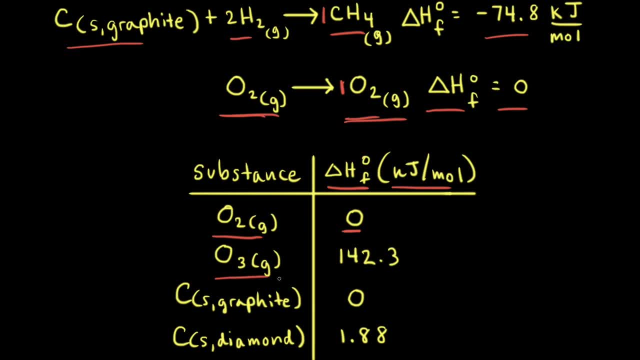 Ozone, which is O3,, also exists under standard conditions. However, it's not the most stable form of oxygen under standard conditions And therefore its standard enthalpy of formation is not zero: It's 142.3.. Sulfite is the most stable form of carbon. 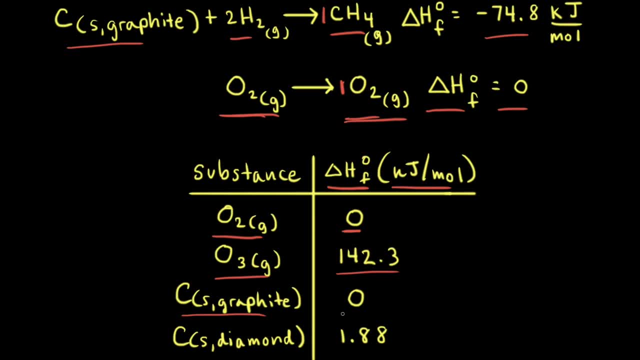 under standard conditions. Therefore it has a standard enthalpy of formation of zero. But of course diamond also exists under standard conditions, but it's not the most stable form, So its standard enthalpy of formation is not zero, It's 1.88 kilojoules per mole. 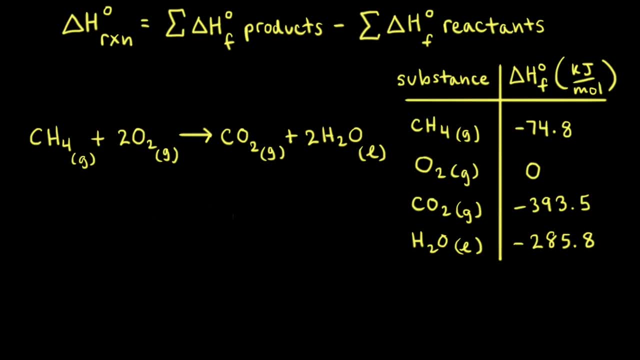 Enthalpies of formation can be used to calculate the change in enthalpy for a chemical reaction. We can do this by using the following equation: The standard change in enthalpy for a chemical reaction is equal to the sum of the standard enthalpies. 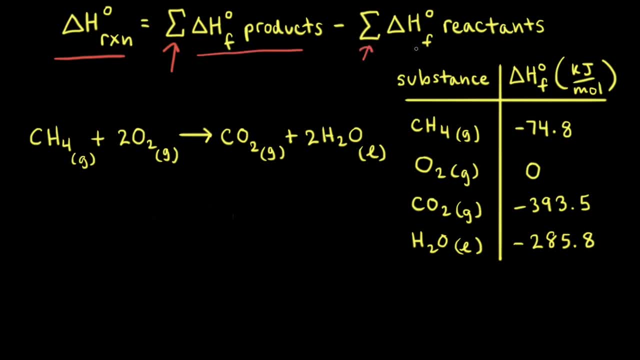 of formation of the products minus the sum of the standard enthalpies of formation of the reactants. Let's say our goal is to find the standard change in enthalpy for the following chemical reaction. So we have one mole of methane reacting with two moles of oxygen to form one mole of carbon dioxide. 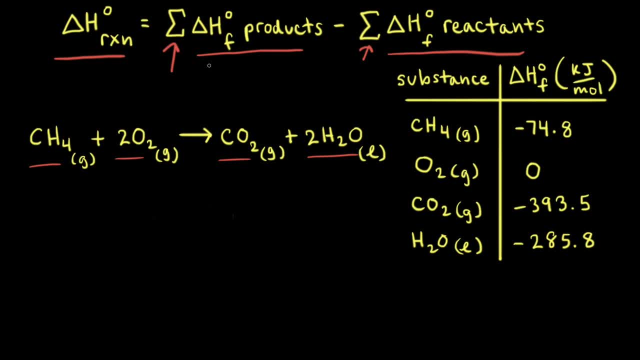 and two moles of water. The first thing we need to do is sum all the standard enthalpies of formation of the products. So if we look at our two products over here, we'll start with one mole of carbon dioxide. So let's go ahead and write this down here. 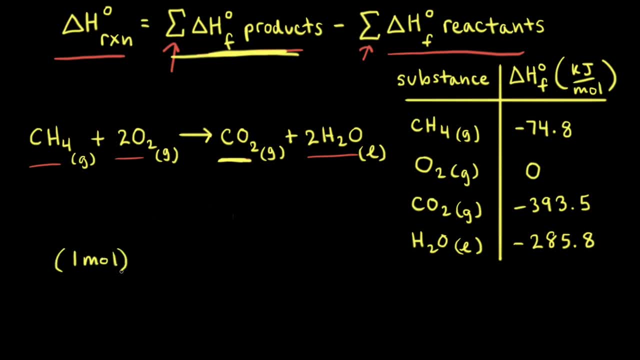 We have one mole of carbon dioxide and the standard molar enthalpy of carbon dioxide we've already seen is negative 393.5 kilojoules per mole of carbon dioxide. So we're gonna multiply one mole of carbon dioxide by negative 393.5 kilojoules per mole. 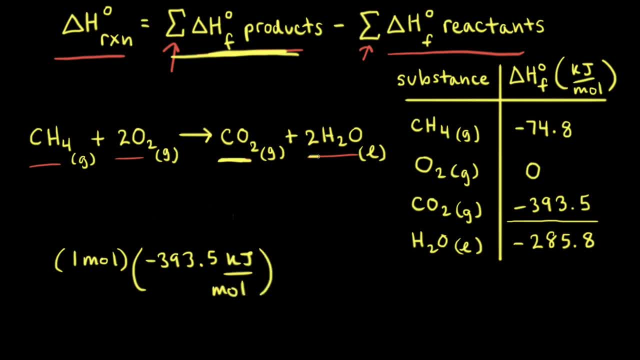 So we get negative 393.5 kilojoules per mole of carbon dioxide. Our other product is two moles of water, So we're going to add this to the other ones. We have two moles of H2O and the standard enthalpy of formation of H2O. 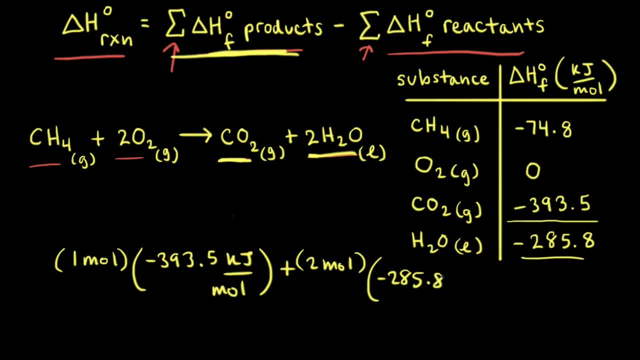 is negative 285.8.. So we're gonna multiply this by negative 285.8 kilojoules per mole, So moles cancel out. so we get negative 393.5 kilojoules And then for the other one moles cancel out again. 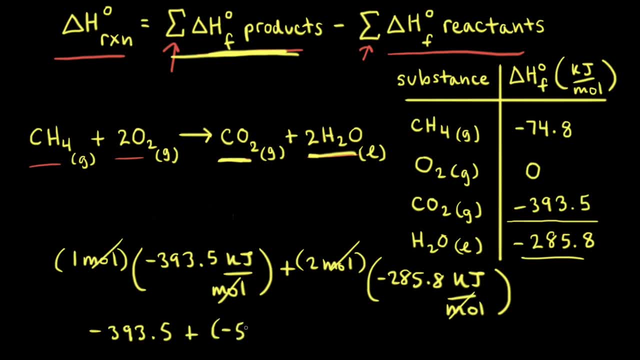 and this would be plus negative 571.6 kilojoules, which is equal to negative 965.1 kilojoules. So that's the sum of all of the standard enthalpies of formation of our products. Next we need to sum the standard enthalpies. 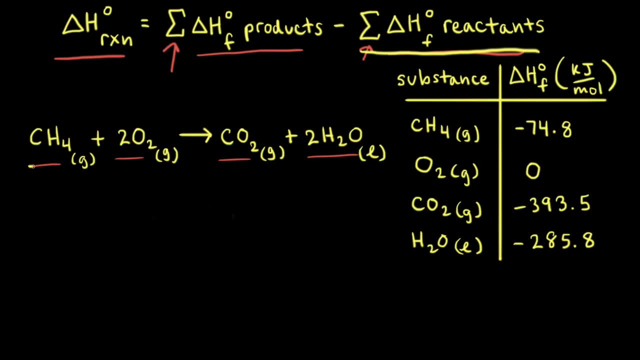 of formation of our reactants. So the two reactants that we have are methane and oxygen, and we have one mole of methane, So let's go ahead and write that in here. So we have one mole of methane. The standard molar enthalpy of formation of methane: 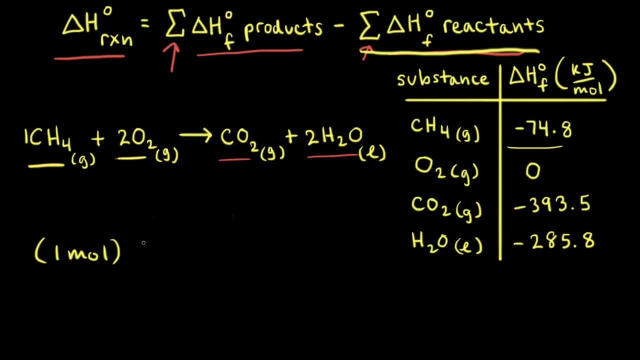 is negative 74.8 kilojoules per mole. So we're multiplying one mole by negative 74.8 kilojoules per mole. Our other reactant is oxygen and we know that. we know that, and we know that diatomic oxygen gas. 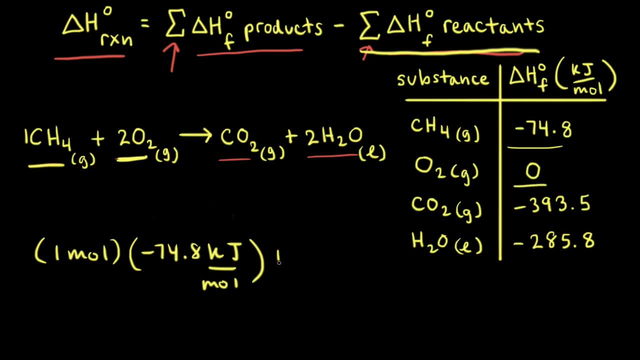 has a standard enthalpy of formation of zero, So we could go ahead and write this in just to show it. So we have two moles of oxygen, but we're multiplying that number by zero, So moles cancel and give us negative 74.8 kilojoules. 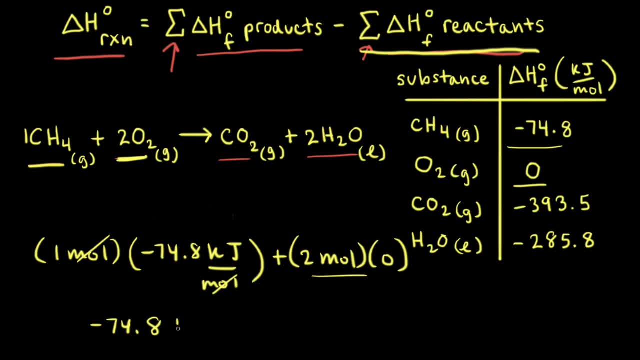 and we're adding zero to that, So negative. 74.8 kilojoules is the sum of all the standard enthalpies of formation of our reactants. So to find the standard change in enthalpy for our reaction we take the summation of the enthalpies of formation. 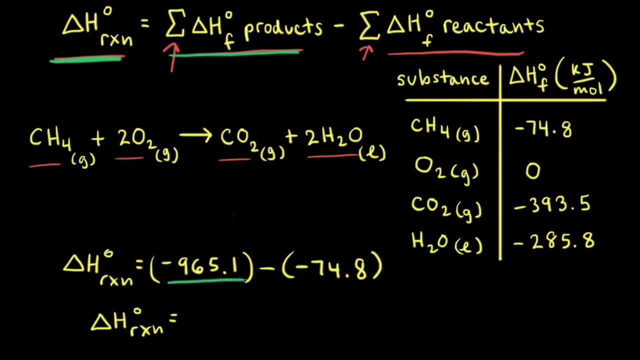 of our products, which was negative 965.1 kilojoules, And from that we subtract the sum of the standard enthalpies of formation of the reactants, which we found was negative 74.8 kilojoules.